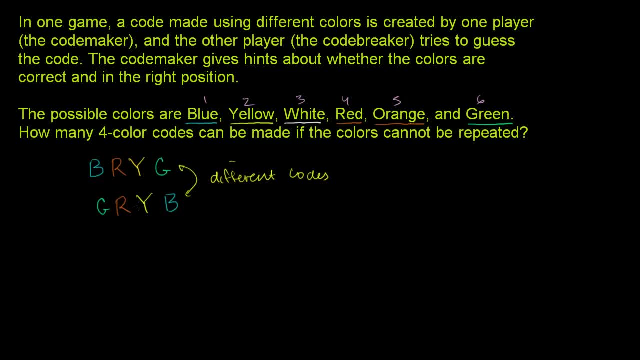 So this would count as two different codes right here, even though we've picked the same actual colors, the same four colors, We've picked them in different orders. Now, with that out of the way, let's think about how many different ways we can pick four colors. 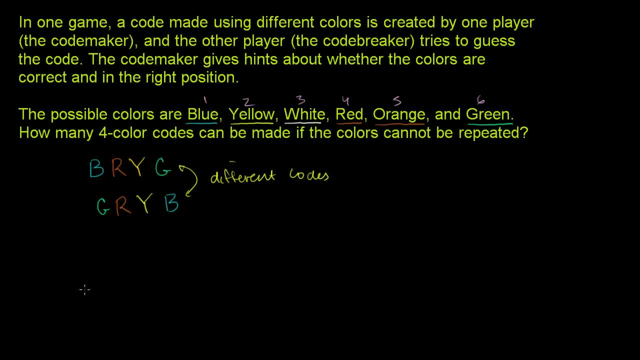 So let's say we have four slots here. We have four slots: One slot, two slot, three slot and four slots, And at first we care only about how many ways can we pick a color for that slot. right there, that first slot. 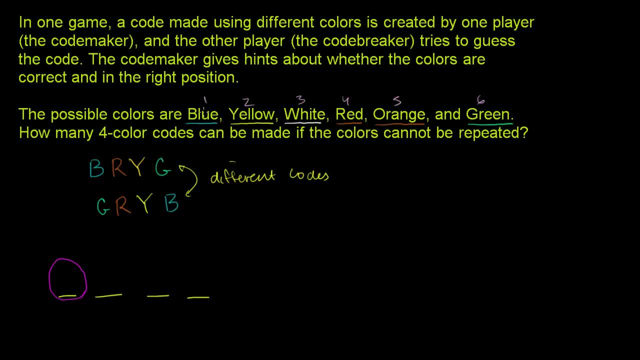 We haven't picked any colors yet. Well, we have six possible colors: One, two, three, four, five, six. So there's going to be six different possibilities for this slot right there. So let's put a six right there. 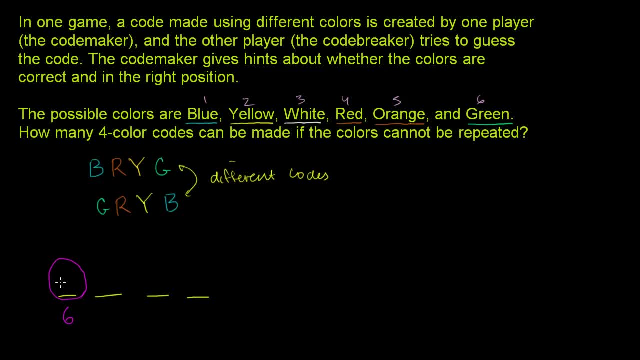 Now they told us that the colors cannot be repeated. So whatever color is in this slot, we're going to take it out of the possible colors. So, now that we've taken that color out, how many possibilities are when we go to this slot, when we go to 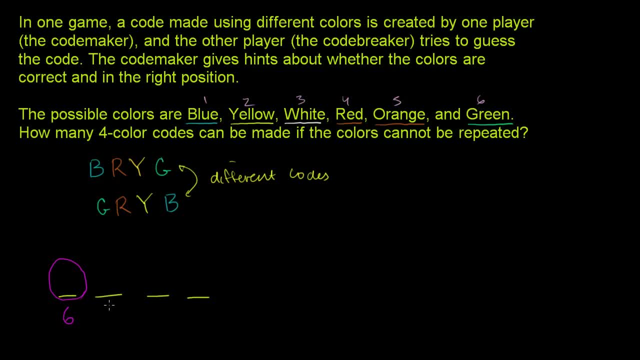 the next slot. How many possibilities when we go to the next slot right here. Well, we took one of the six out for the first slot, so there's only five possibilities here, And by the same logic, when we go to the third slot, we've 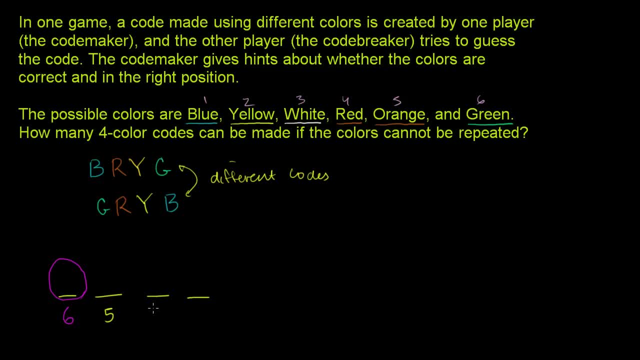 used up two of the colors already, so there will only be four possible colors left. And then for the last slot, we would have used up three of the colors, so there's only three possibilities left. So if we think about all of the possibilities, all of the 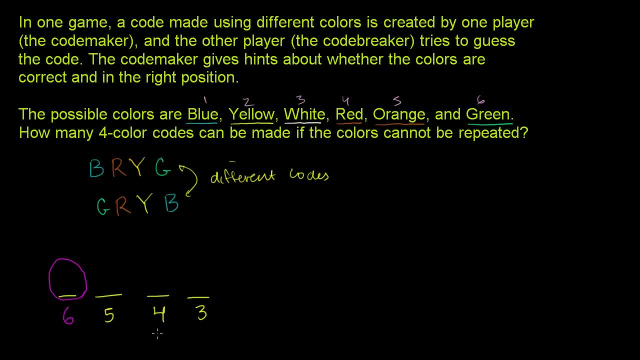 permutations. and permutations are when you think about all the possibilities And you do care about order, where you say that this is different than this, this is a different permutation than this. So all of the different permutations here, when you pick four colors out of a possible of six colors, it's 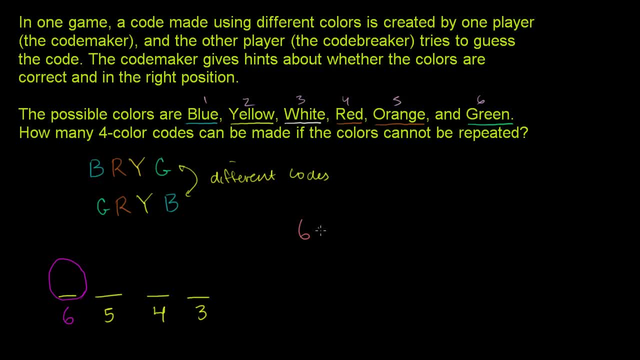 going to be six possibilities: for the first, one times five. for the second bucket, times four. for the third, or the third bucket, or the third position, times three, So six times five, is 30 times four, is times three, so 30 times 12.. 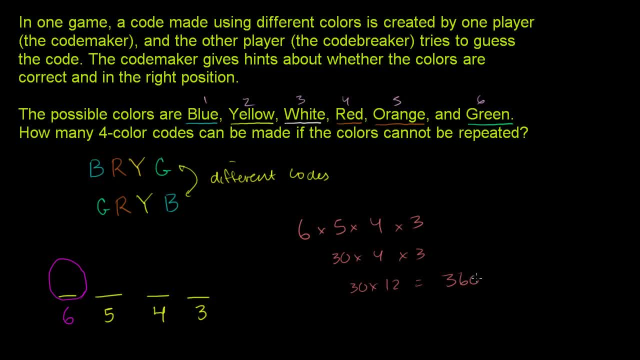 So this is 30 times 12, which is equal to there are 360 possible four color codes.